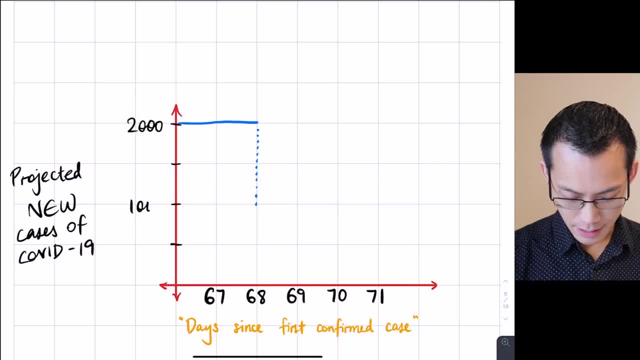 So I'm going to have 1,000 time, like so, and 1,000 is going to be here on my vertical scale. So from day 68 onwards I'm going to have- let's go in blue now I'm going to have a gradient of 1,000. 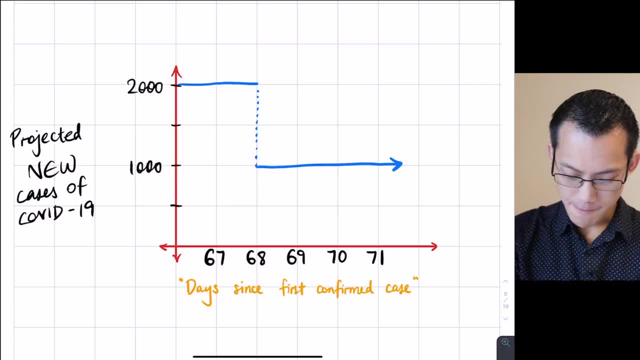 There we go. That's what the shape of the graph is. Now, this is a weird-looking graph. We call it a step function because it looks like a set of steps. not that you need to know the technical name, But this thing's weird. 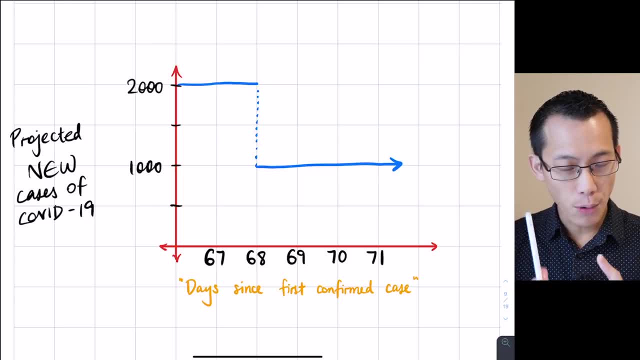 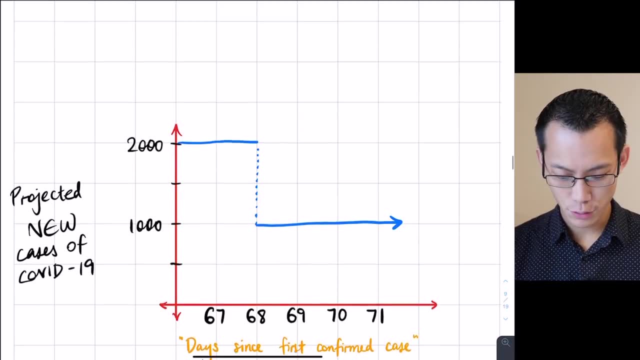 It's sort of brutal, It's broken into pieces, But we can still understand it and, importantly, we can still answer that original question from this different perspective of a derivative. And let me just repeat that again, We're going to go back to this original question. 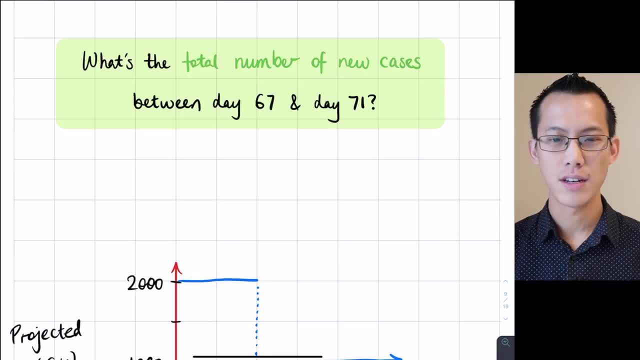 What's the total number of new cases between day 67 and day 71?? We can answer that same question on the basis of this new graph. Just imagine- just forget about that earlier graph that we did before- Suppose this was the only graph that was presented to you. 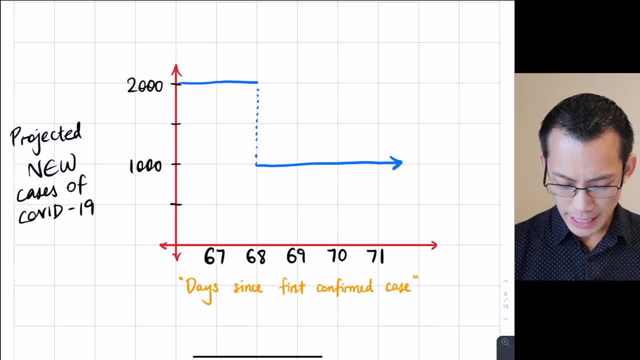 If you want to work out how many new cases there have been over that time, you would do this in chunks, right? You'd say, well, from day 67 to day 68, that's this sort of time period. here there's a single day that passes and during that day 2,000 people are diagnosed. 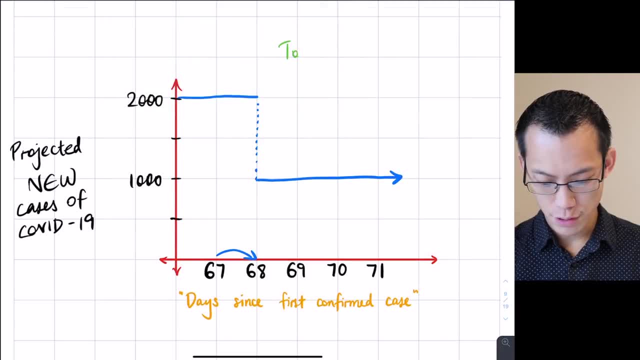 So let's do some working here. If I said the total number of new cases, I should say new cases. sorry, I said it, but I forgot to write it: The total number of new cases. well, for starters, there's going to be that one day where 2,000 people are diagnosed, 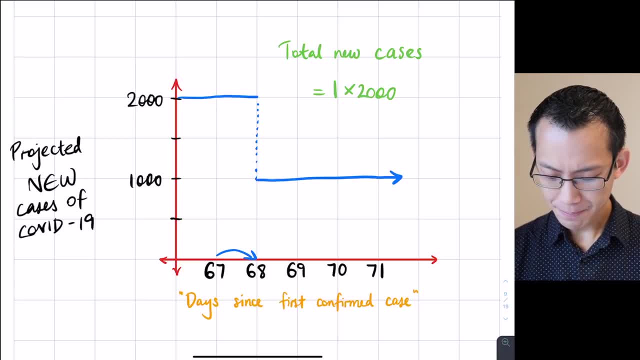 That's from day 67 going over to day 68.. But then there's this new part of it, right As I go from day 68 to 71 across here, and then I stop there. Sorry, my arrow's gone just slightly too far. 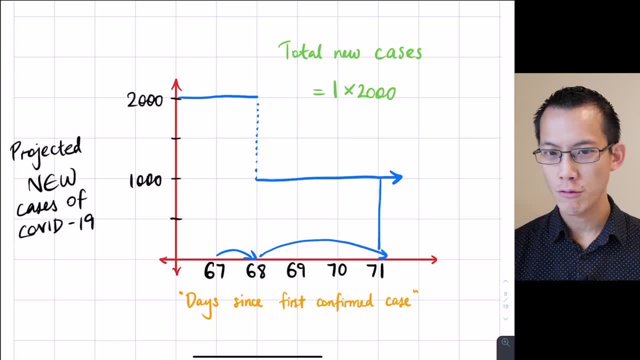 Here I've got three days that pass, And then there's a new rate at which new cases are diagnosed. Three days and each day, just like you told me, there's 1,000 new cases diagnosed. So I'm going to add on to that one lot of 2,000, one day with 2,000 cases per day. 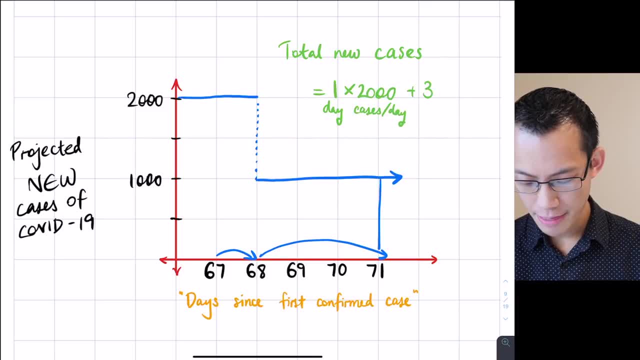 I'm now going to add on to that an extra three days where I get 1,000 cases per day. I've still got 3,000.. the same units there. I'm going to cheat a little bit and be lazy, sorry guys. 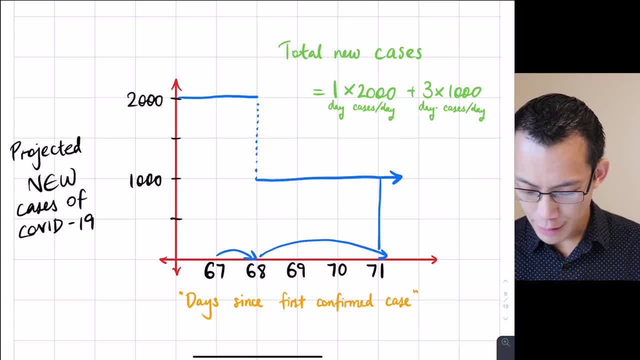 Okay, there we go. So I've got three days there at a slower rate and so, thankfully, hopefully, things will improve from here. Now the numbers again, like before, are simple, right? One lot of 2,000 gives me 2,000, three lots of 1,000. 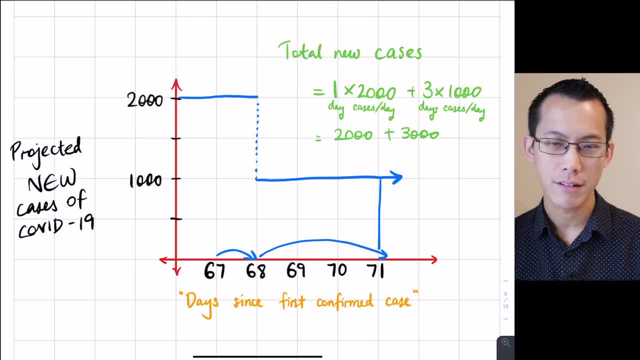 give me 3,000 and, much to our relief, this is exactly the same answer that we got before In mathematics. if we approach a problem from a different way, we shouldn't expect to get a different answer. we should expect to confirm the previous answer that we got now. what does this tell us? What can we learn? 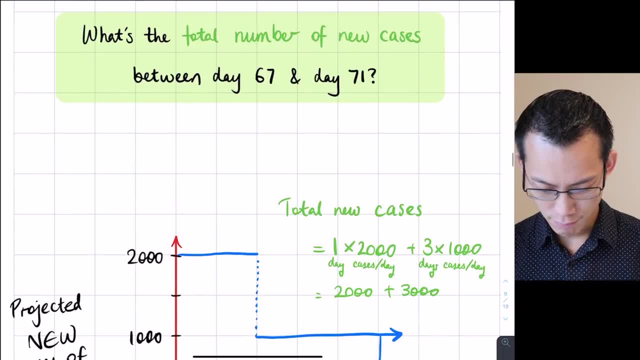 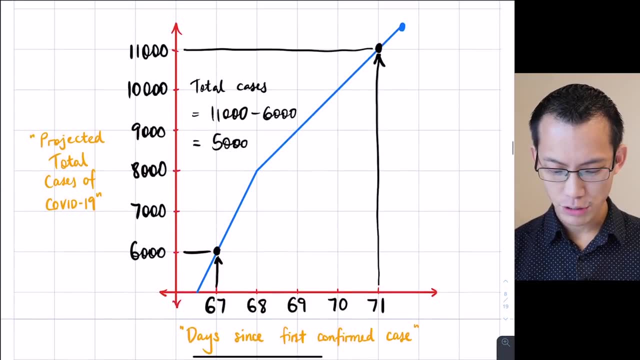 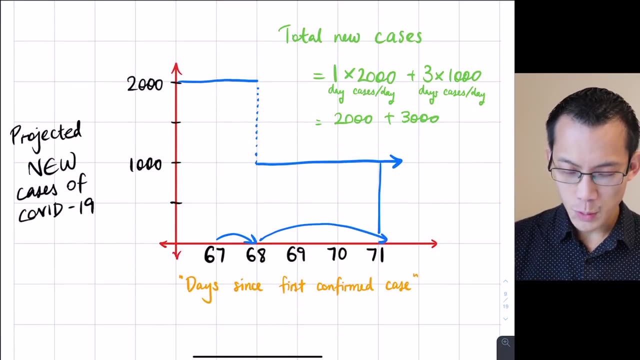 from looking at the same situation- total number of new cases- between this particular time period- and looking at it from two different perspectives. Initially we looked at it from a sort of total, accumulative sense and we did this subtraction. and then here what we did was we had a look at it from the 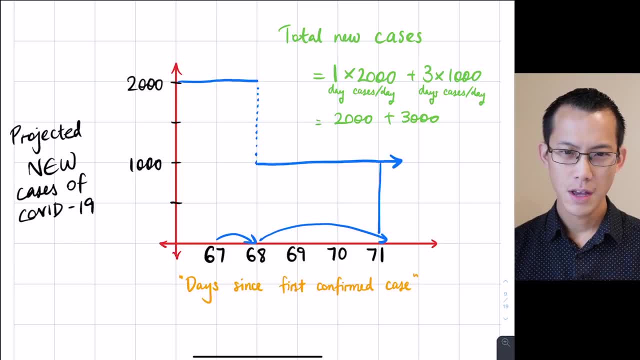 perspective of the derivative, from the perspective of the resolved subject. this self-finding will really help us understand how we should rate of change. What this tells us is that really, these two things are one and the same. If I only gave you this derivative graph, you could work it out by saying: oh, 1 times 2,000 actually. 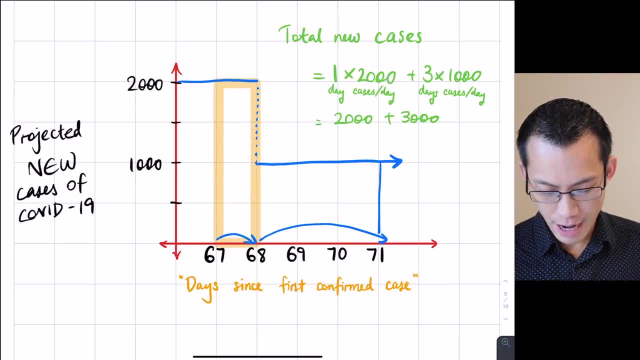 represents. I'm going to draw a rectangle in here- this area at the top right, That's the 1,, which is the width, and the 2,000,, which is the height, And then, in addition to that, I also have this: 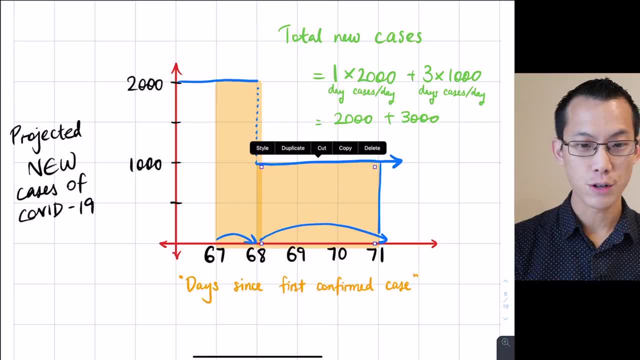 other guy over here- another rectangle which is 3 wide and it's 1,000 tall. I'm calculating like we looked at last lesson, the area under the curve. Now, in this case, the area under the curve. 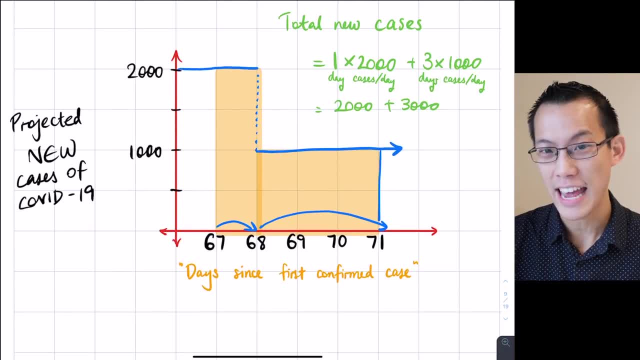 is really easy to work with because they're nice, regular shapes. They're rectangles, the easiest kind of shape to evaluate the area of. But often, in fact for years now, we've been dealing with functions that don't have nice, neat curves like this. They're all wiggly and wobbly and we don't. 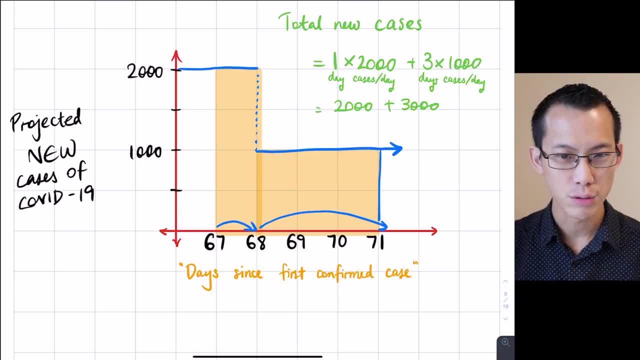 have nice neat curves like this. So we've been dealing with functions that don't have nice length times, breadth or base times height on 2. for those triangles we were having a look at last time We've got really complicated shapes that we don't simply have a formula for. So in those 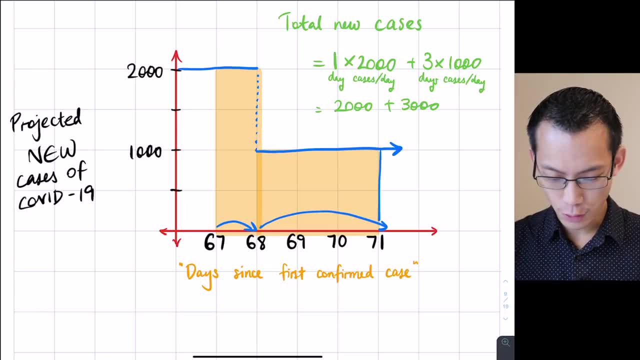 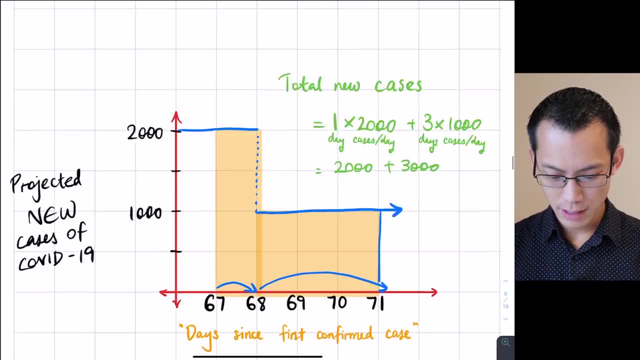 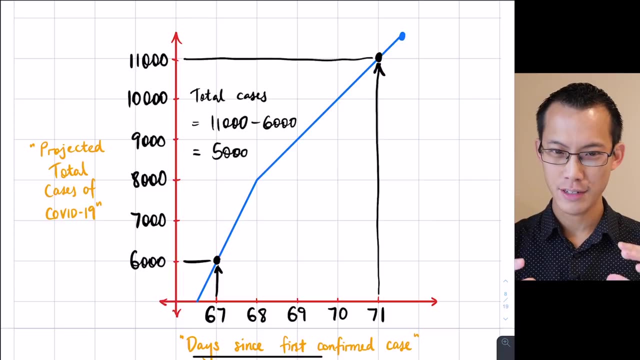 cases. if I asked you for the area under the curve of a graph like that, how would we do that in the absence of an area formula, like we learned in year 7 and 8?? And the answer is by having a look at where we started, By going up, instead of going from this graph and then differentiating to go. 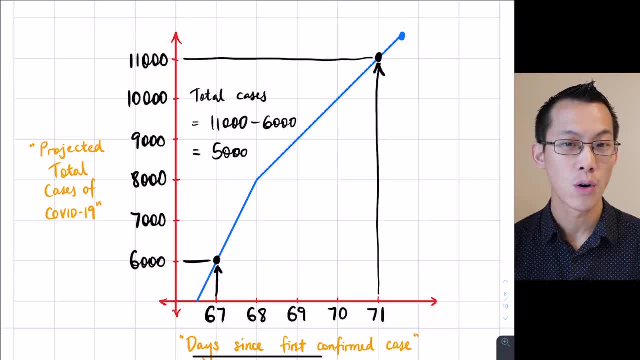 down. we know that the reverse of that process, this is what we call integration, right, Anti-differentiation. if you might remember, that's how we first introduced it. So if you've got this weird wobbly looking curve that it's difficult to work out, the 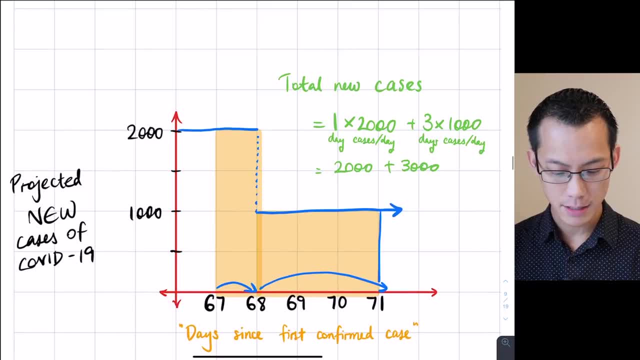 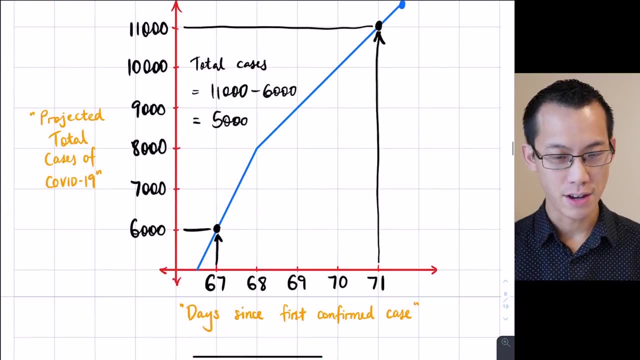 area of you can't just break it into neat and easy rectangles like this. then, instead of trying to break it into such areas, you integrate. That will take you to this curve, and then you simply take the difference between one value and another. You will end up with this same solution. So 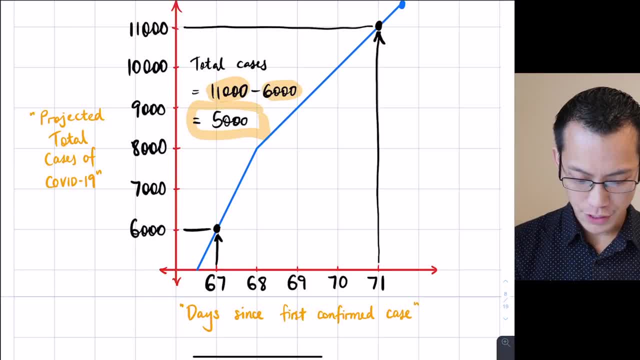 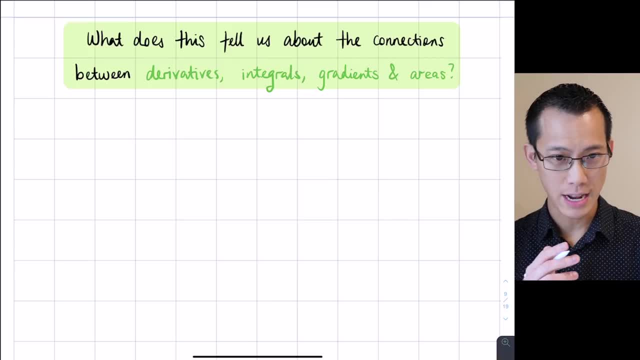 underneath where you've put those two graphs. let's try and capture what we've just said in some of the notation that we've already been using. okay, Underneath here, what does this tell us about the connections between everything? Well, I was interested. remember, in total change That 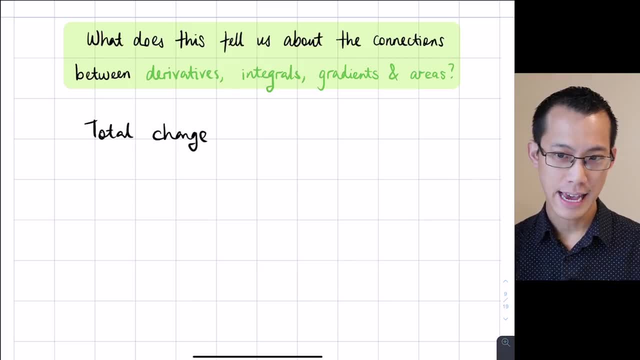 was the question I was asking about these COVID-19 cases, and we looked at it in two different ways. The first way was to say, well, just have a look at where you ended and subtract that from where you started. So if I have a thing like this, I'm going to subtract that from where you started. So 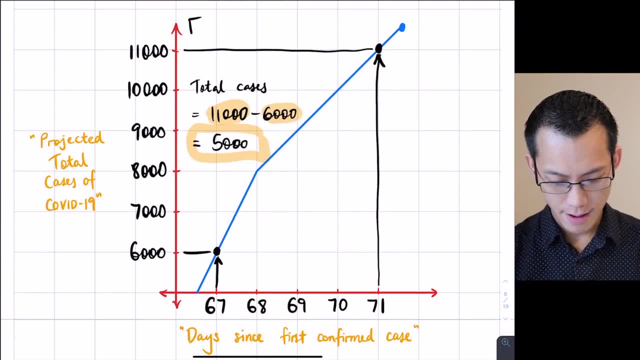 if I have a thing like this, I'm going to subtract that from where you started. So if I have a thing like this, I'm going to subtract that from where you started. So if I have a thing like this, let's call this guy F of x capital, F 11,000 and 6,000.. Where did I get those numbers from? The 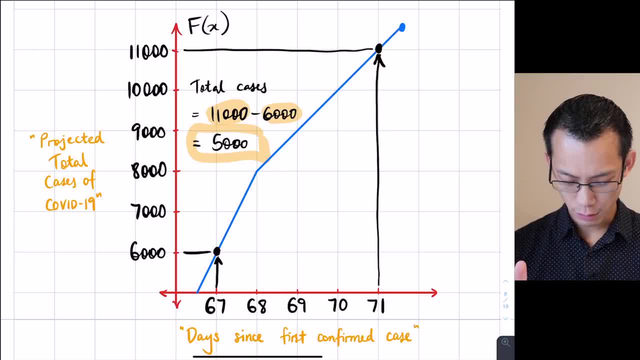 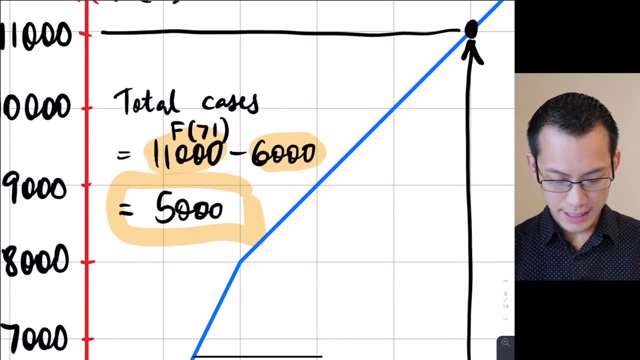 answer is: I looked at the horizontal axis, I looked at the appropriate days- 67 and 71, and then I went up to the graph to see where that matched right. In other words, that 11,000 was really F of 71. That's where I got that value from, And the 6,000 was really F of 61. So 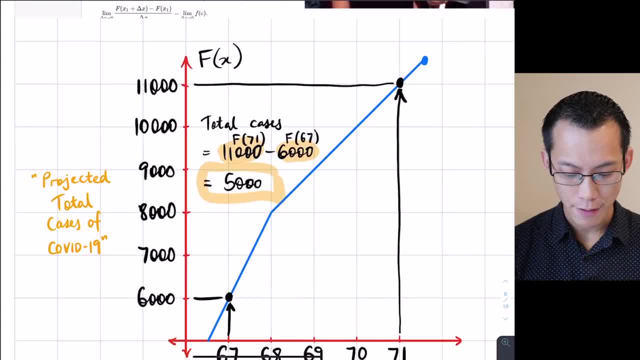 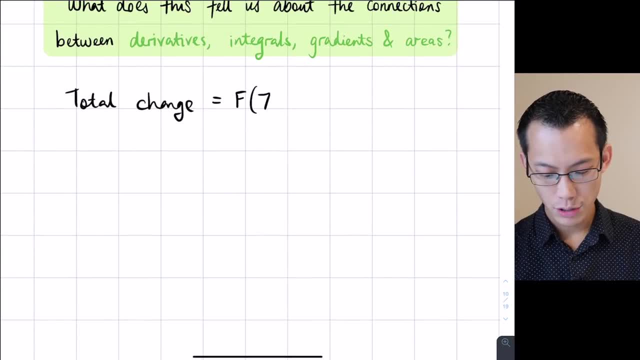 67. that's where I read it off of the graph. I got those vertical values, so now I can take that together and write. well, the first way that we calculated this was: look at your state at the end and subtract that from your state at the beginning. you'll work out the difference and you'll get your answer, which we 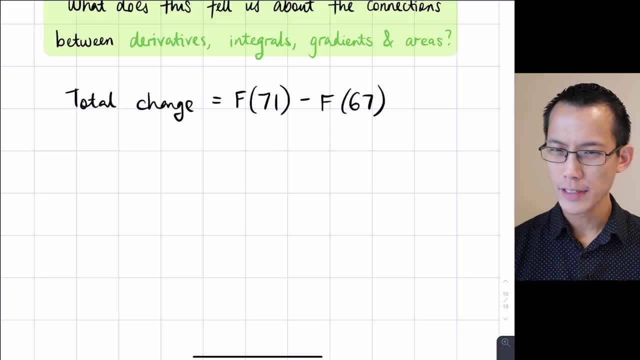 worked out was 5,000, but you can equivalently look at it from the perspective of a rate of change. that was the second graph. I'm going to use some colors here to help me. a rate of change, and then you multiply that by how much. 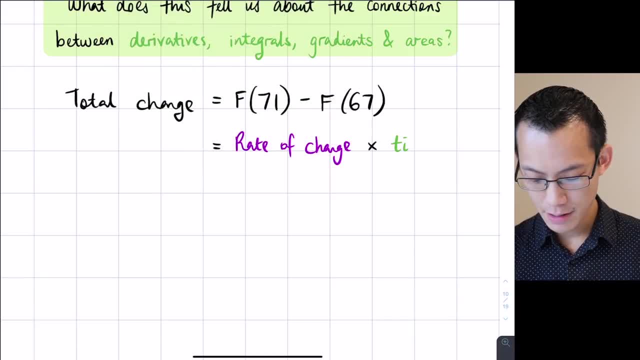 time you spend at that particular rate. so, for example, we had a rate of 2,000 per day for one day and we multiply that together and we included that with a rate of change of 1,000 per day for three days, and we did that over and over. 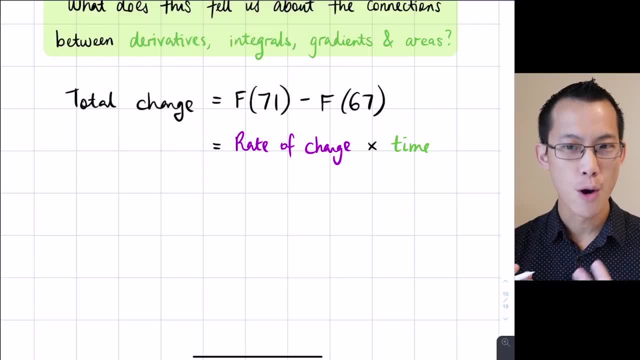 again now to say that, to say we we do that over and over again for all the different parts of our graph. we use this notation that we introduced before this elongated s: we're taking the sum of all of those different areas. in our case it was pretty easy, just two rectangles from: 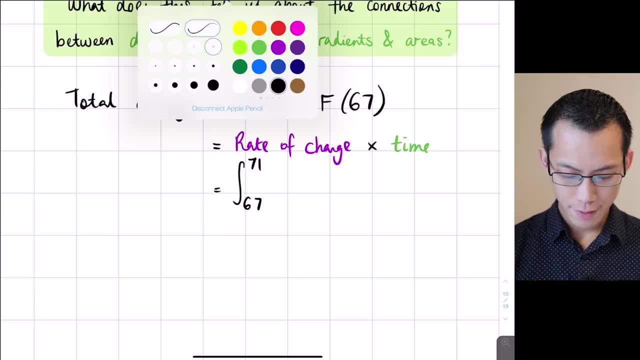 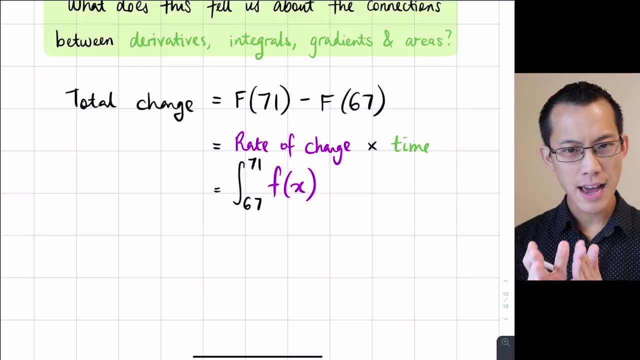 67 to 71 of number one, our function, which is the rate of change. that's why I'm using these two colors here to separate them. and then our time was on the horizontal axis. remember that. so the change in time. we would use the letter D. 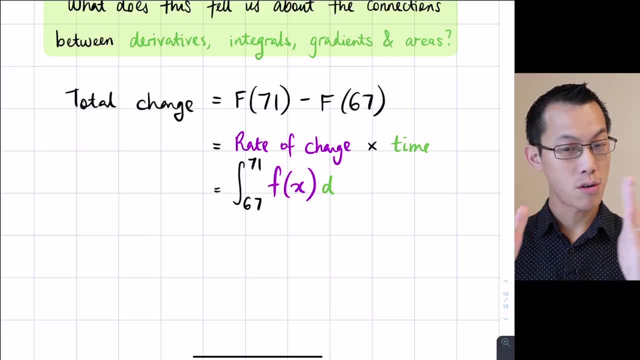 to indicate change, like Delta, and because it's on the horizontal axis, we would say, well, that's, that's an X value, right? so this is the familiar kind of notation that you've been seeing for a while in differential and integral calculus. now, all of this is particular to this specific example. day 67, day 71. 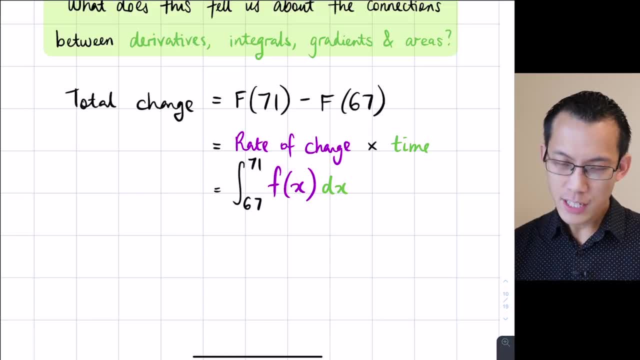 and those values of 11,000 and 6000. but this whole idea of looking at a function, looking at its integral to working out, to work out area. this is always true, no matter what numbers you throw at it, and that's what the fundamental theorem of 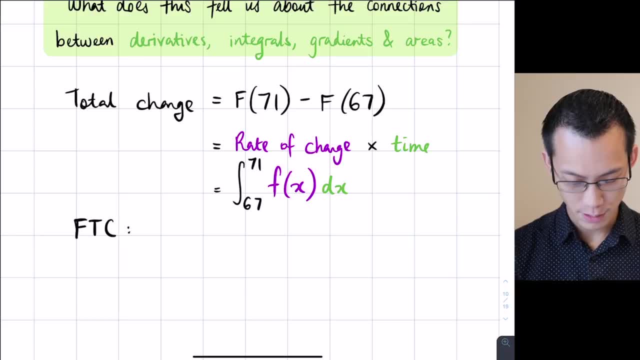 calculus is. I'm just going to write F, T, C, because those words are too long for me to write. The fundamental theorem of calculus tells us this right If we want to work out the sum of all the areas from some starting point to some ending point.